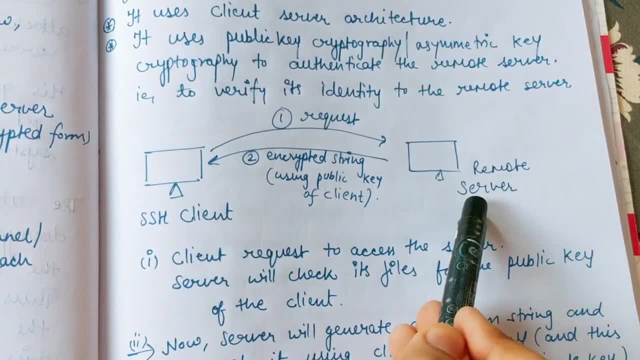 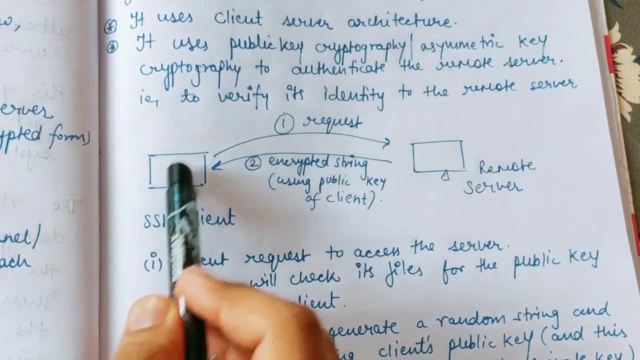 our diagram. Suppose we have a SSH client- Okay- And we have a remote server. We want to access some files from this server, or if we want to get some files right. So what will happen is, first of all, we will send a request to this remote server, Okay, So 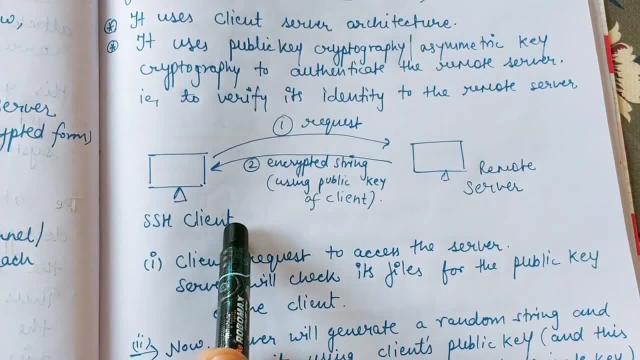 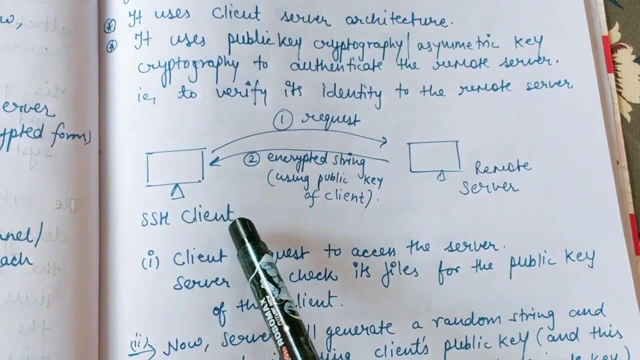 in order to know that, yes, whether we are the authentic user or not. Okay, So what will happen is this remote server will first of all check our public key- Okay, Because public key is known to everyone, right? So, guys. then afterward, the server will check the. 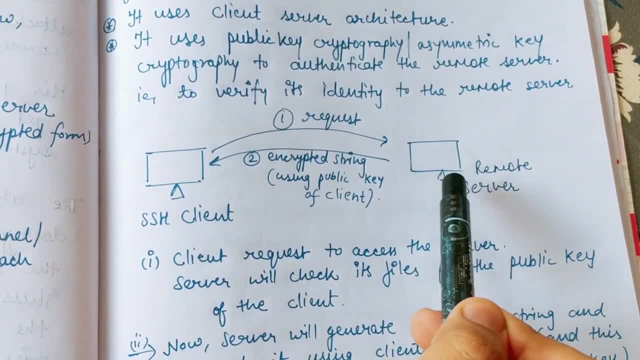 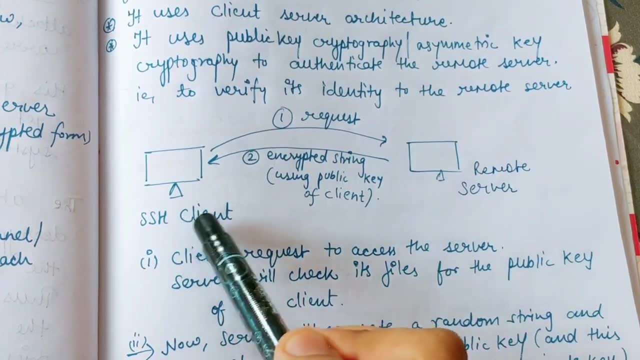 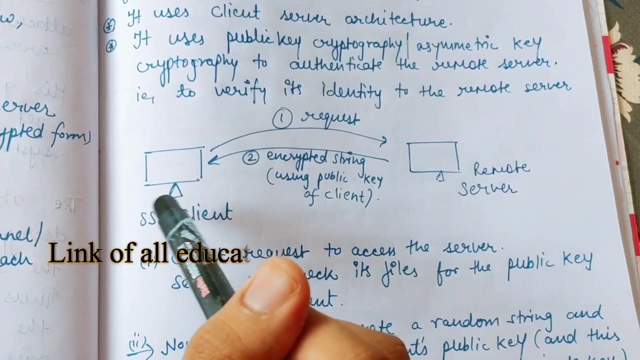 public key in its files. right Afterwards, when the public key is found, what remote server will do? This server will create a random string and then encrypt it using the public key of this client. Okay, Because if we will encrypt it using this public key of this client, then only this client will. 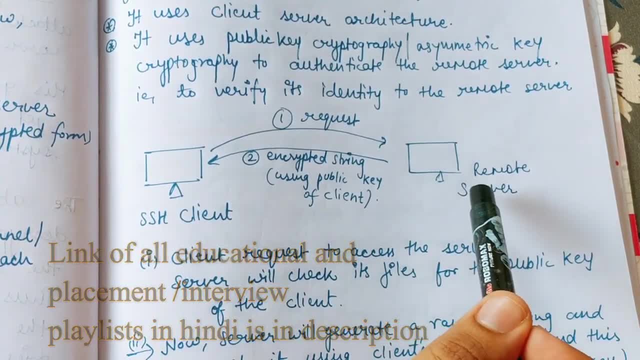 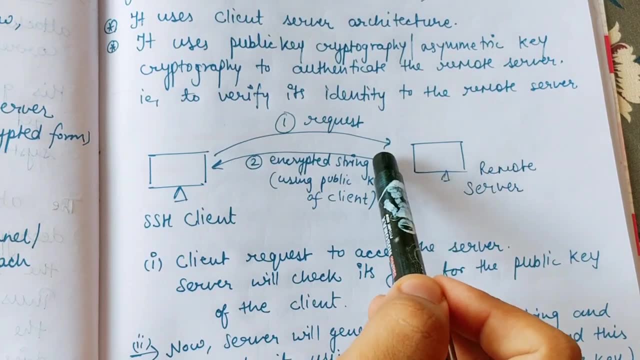 be able to decrypt it. Why? Because if we encrypt something using the public key, that can only be decrypted using the private key of that particular user right. So that's why this server will generate a random string and encrypt it using the public key of this. 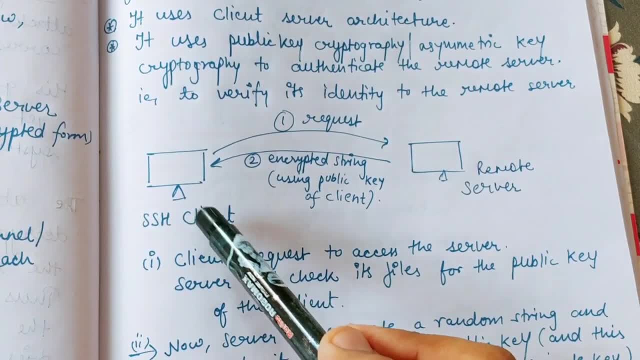 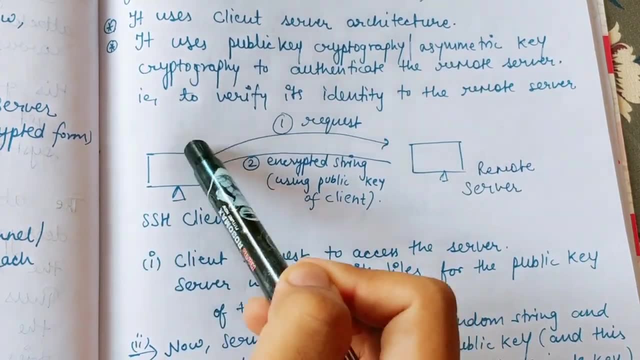 client. Then guys, this client will decrypt that string by using its own private key. Okay, Because private key of that user is only available to this particular user only. Okay, Because attacker cannot have a private key Right, So as clients will simply decrypt that. 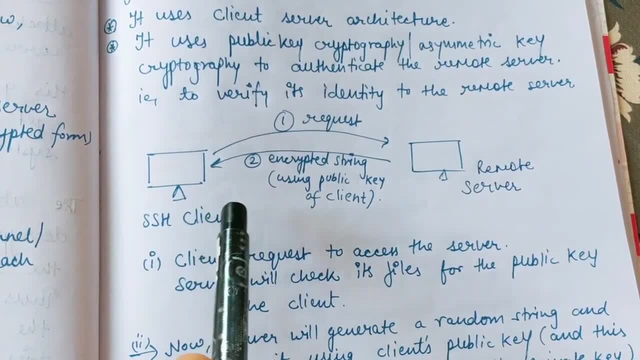 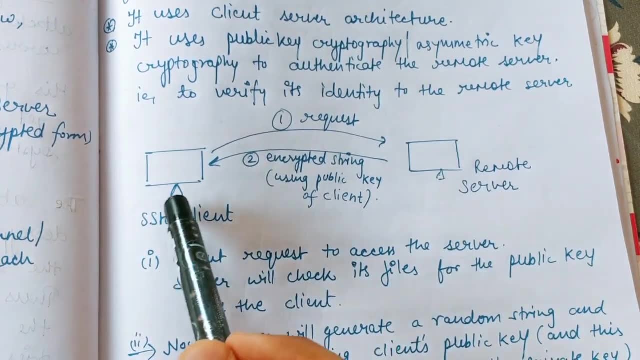 message, okay, By using its own private key. then afterwards, when the client will get that particular string, this client will acknowledge the remote server about it. Okay, That is, the client will send this message to the server. Okay, And then the server will check that. 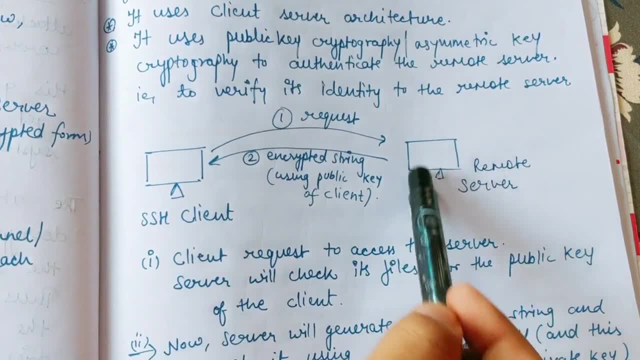 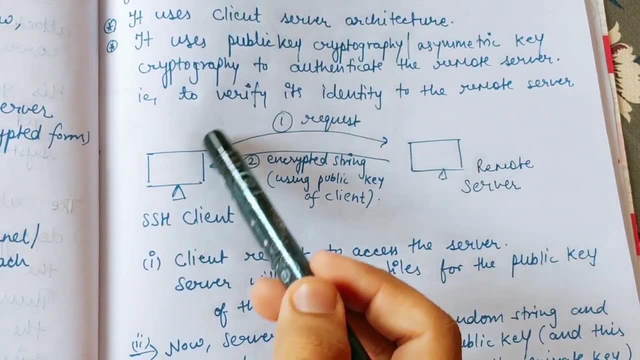 yes, this was the message which I sent to the client, and in this way authentication is achieved right. so now the server also knows that the user is authentic, so what happens is a tunnel is created in between them and then simply transfer of data can take place securely. we can send our data by: 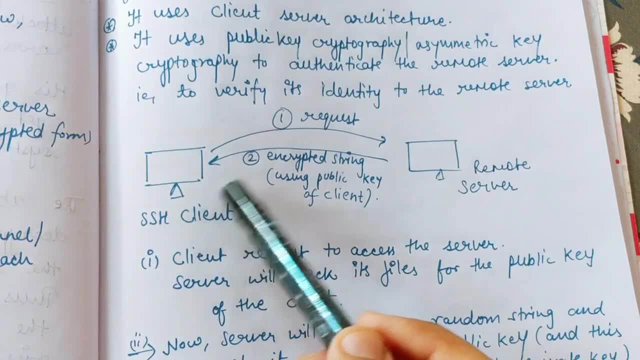 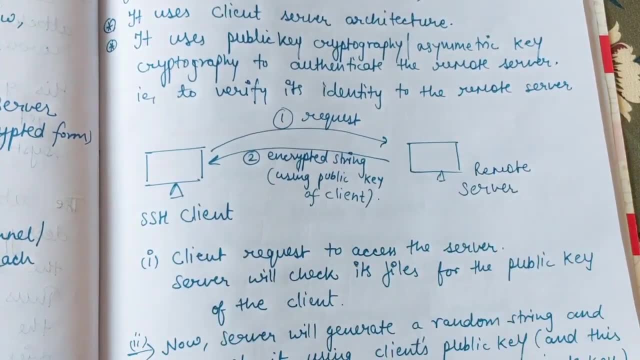 using encryption technique and simply no one can attack our data. okay, no attacker can come in between. so this is the beauty of ssh protocol: that we will get the security over our unsecured network. now, guys, the same thing i have over written over here so that you can write in. 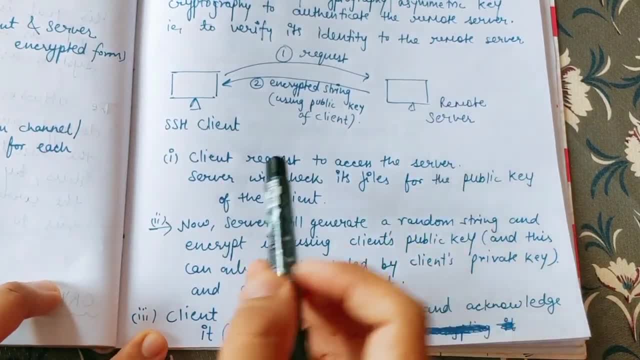 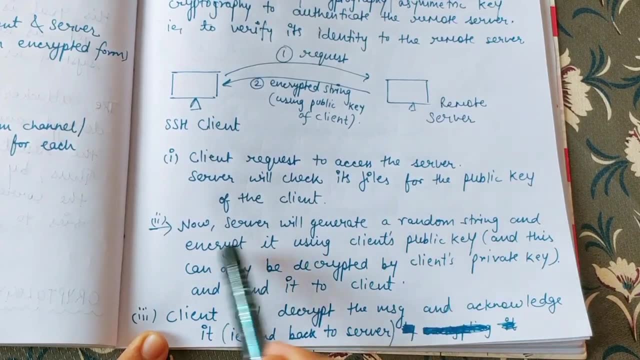 exams. also, if you want to write so, client will request to access the server. right, then server will check its file for the public key of the client now. after that, server will generate a random string, okay, and then encrypt it using the client's public key and afterward the client will decrypt it using its own private key. 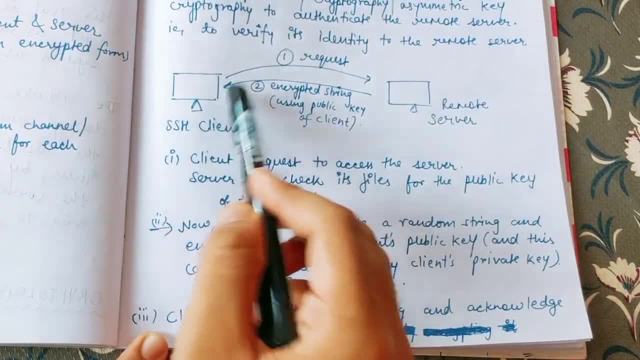 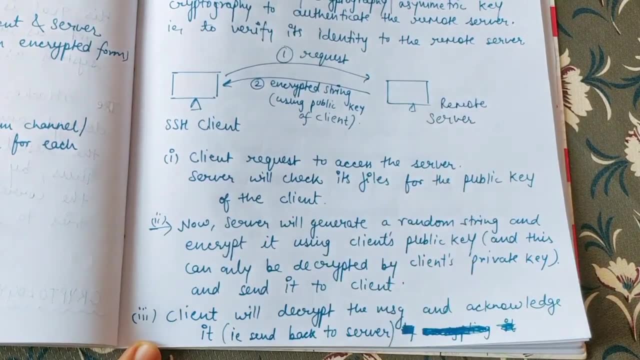 and send it to the client. right then the remote server will send that stream to the client. encrypted steam to the client is straight now. third part client will decrypt this message and acknowledge it to the server and then afterwards the server will know that, yes, this is the authentic. 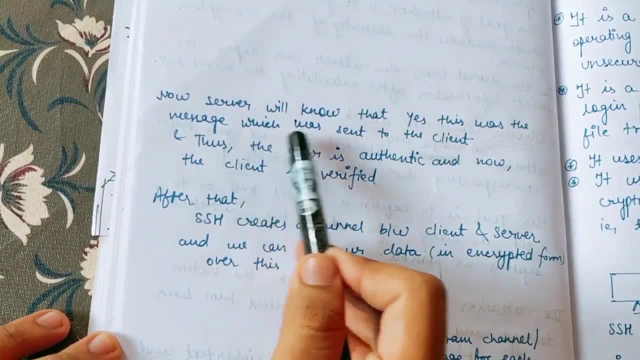 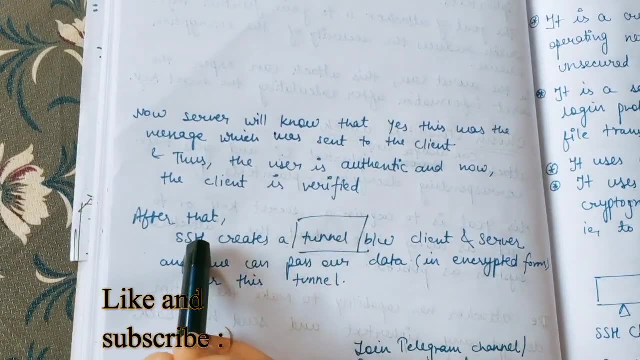 person. so now server will know that, yes, this was the message which was sent to the client and thus the user is authentic. or we can say: the user is verified now, okay. so guys, now, after that, SSH creates our tunnel between the client and the server and we can pass our data in a secure manner. okay, by. 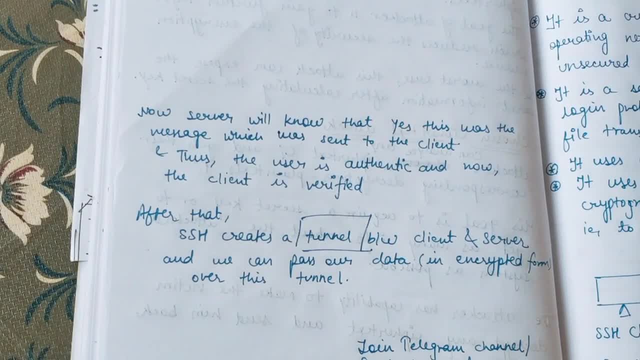 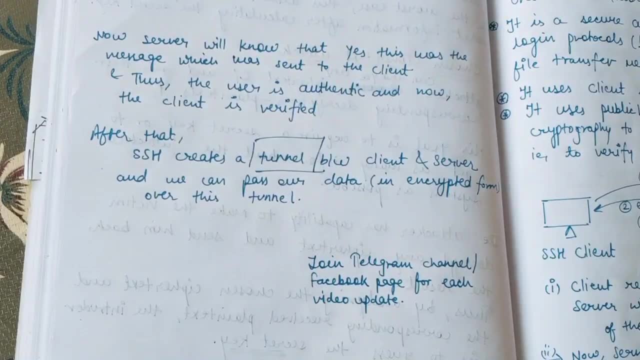 using our encryption techniques. so basically, we can see that no attacker will be able to attack our data when we will use our SSH protocol. okay, it provides us the security over an unsecured network. guys, you can also join my telegram channel or my facebook page or even my Instagram handle for regular 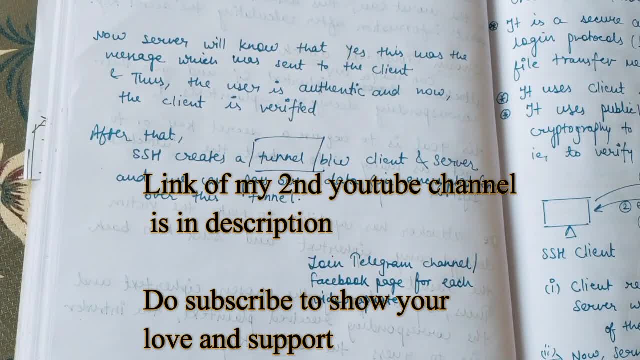 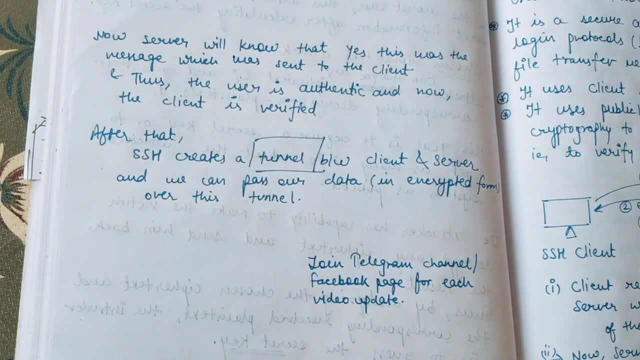 video updates. okay, you will get the link in the description and you will also get the link of my second channel in the description. on that channel I upload videos in Hindi of various subjects and placement related videos. if you know Hindi, you can join that channel also. on that channel I have already uploaded. 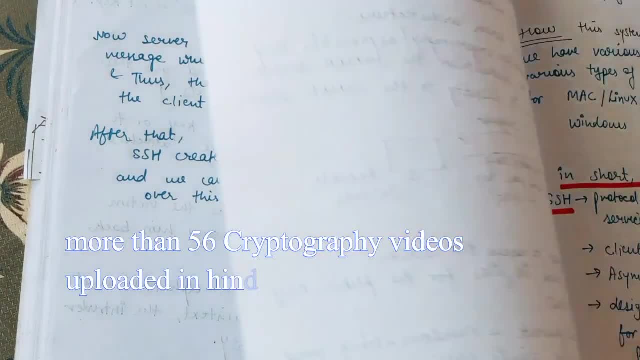 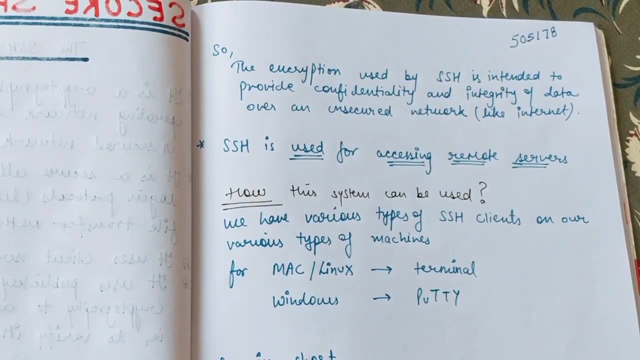 cryptography series. almost 55 to 56 videos have already been uploaded. you can check that. okay, you will get the best explanation in Hindi. so the encryption uses are very simple and it is very easy to understand and it is very by. the SSH protocol is intended to provide confidentiality and the data 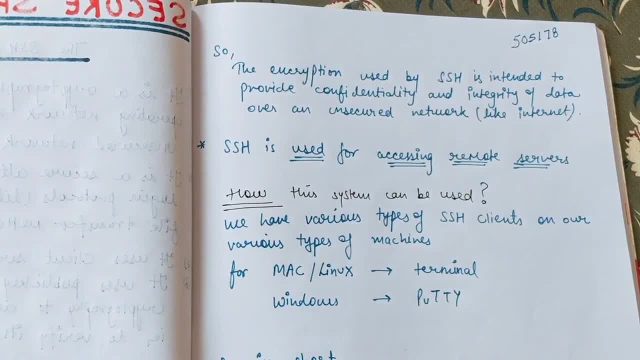 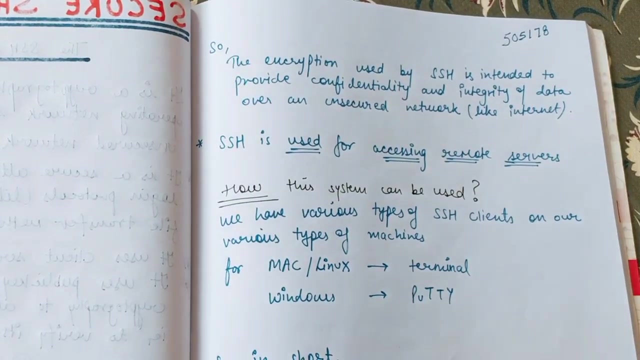 integrity over an unsecured network. okay, like internet. so no attacker will be able to attack our data. the information will remain confidential, but only between me and my server, right, so SSH is used for existing the remote servers, as we have seen in the previous diagram. right, we are simply able to access our remote. 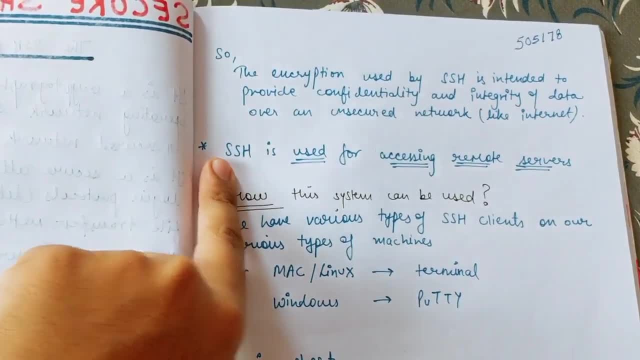 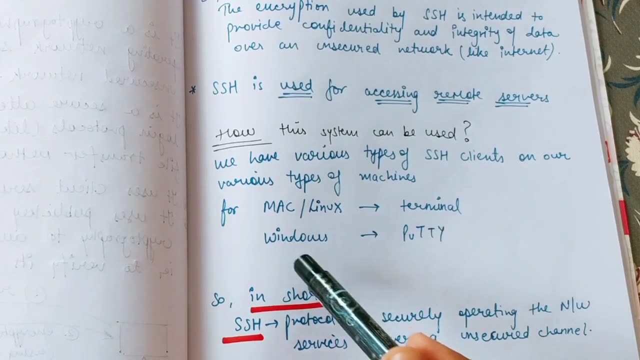 server and we can fetch the files, whichever files we want, by using the SSH protocol. now how this system can be used, guys: if you have Mac or Linux, then terminal will act as your client, as such client, and if you use Windows, we can use various Software's, but one of them is beauty.